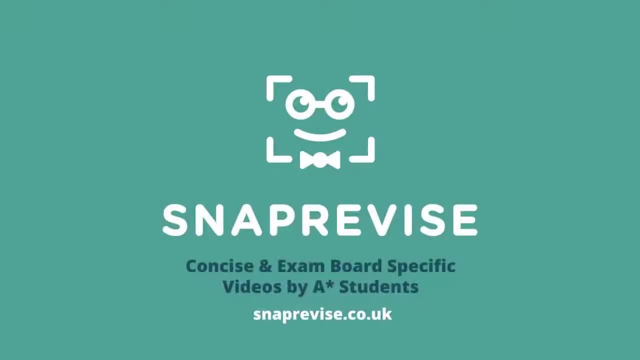 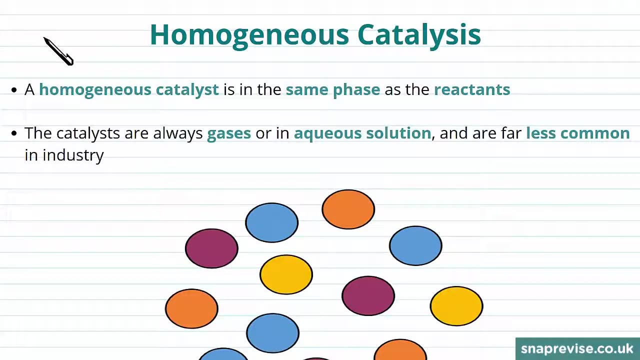 Hi guys, in the last part of the video we looked at heterogeneous catalysis using transition metals. We're now going to look at homogeneous catalysts, and remember that homogeneous means that they are the same phase as the reactants in the reaction. The catalysts with homogeneous 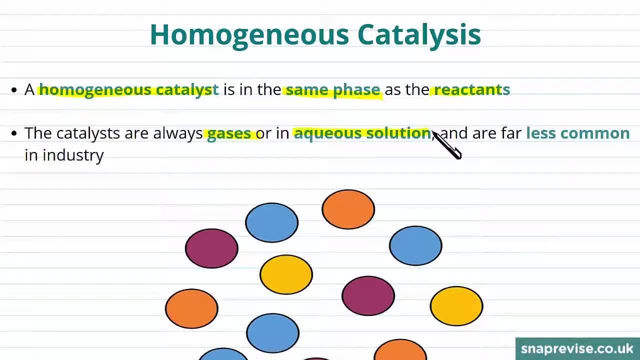 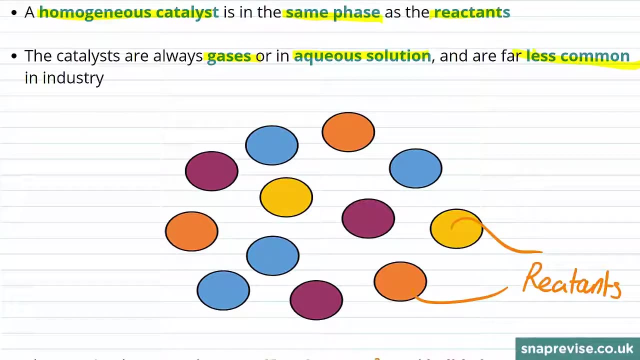 catalysts are always gaseous or in aqueous solution because we can't easily have lots of solids reacting together. Using homogeneous catalysis at all is far less common in industry because if all of our reactants, products and the catalyst itself are all in a mixture, 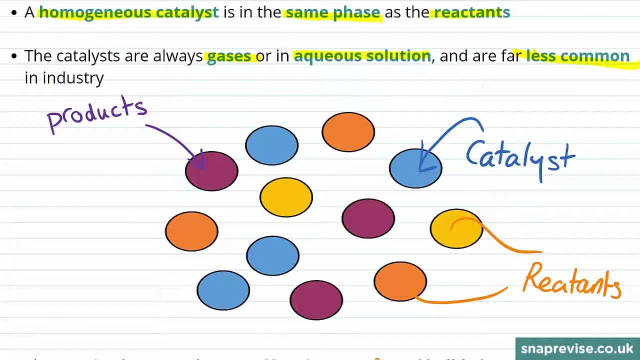 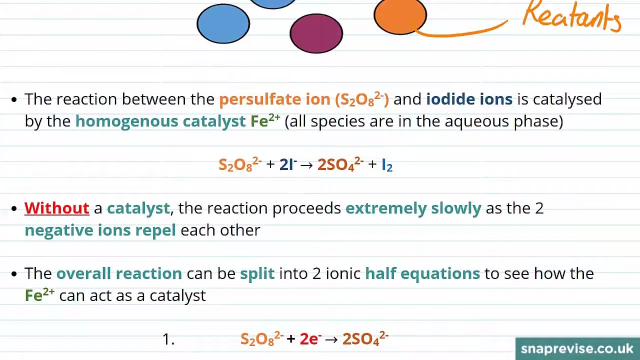 where their gaseous or aqueous particles are all jumbled together. it's very hard to remove the products from the catalyst and the reactants easily to purify what we want to get out of the reaction, Which is why it doesn't tend to be used in industry. We can still study examples of these. 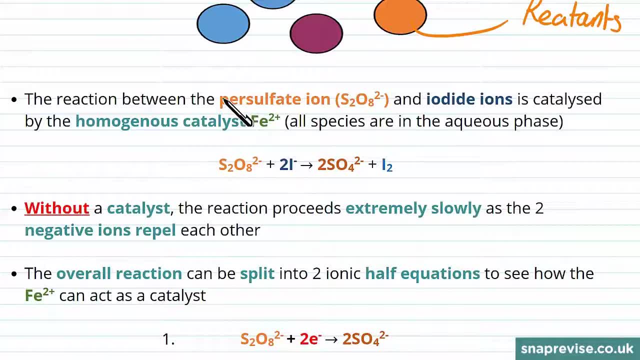 catalyst reactions though. so we're going to look at the persulfate ion S2O8 2- reacting with iodide ions, and this is catalysed by ion 2+. All of these species are in aqueous phase, which makes the ion 2+ a homogeneous catalyst, The reaction we want to catalyse. 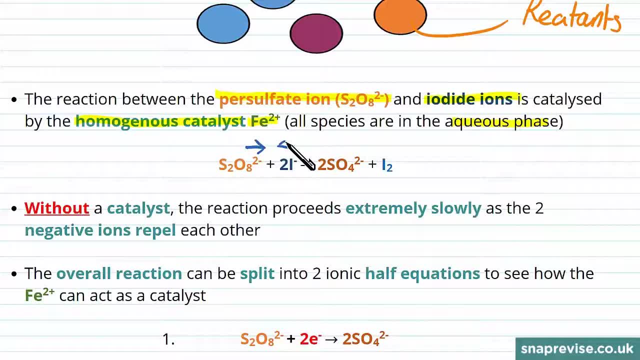 is between the persulfate ion and the ion 2+, But to make this happen, two negative ions have to come together, and this makes the rate of reaction extremely low. Instead, we want to separately react the iodide ions and the persulfate ions with the ion catalyst, and in this way they don't have to interact. 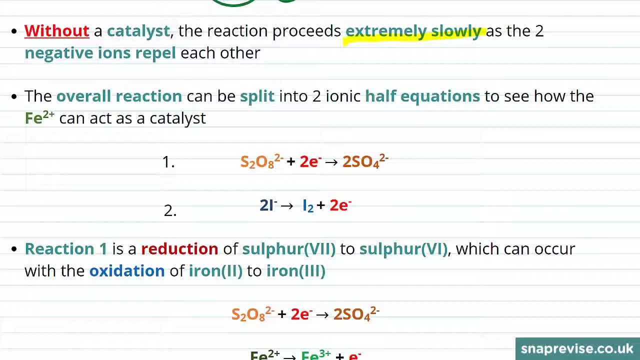 with each other. So we can split the overall equation we've just seen into two ionic half-equations that show either the reduction or the oxidation of each of the reactants. Here we have the persulfate ions gaining electrons. so this is reduction and here 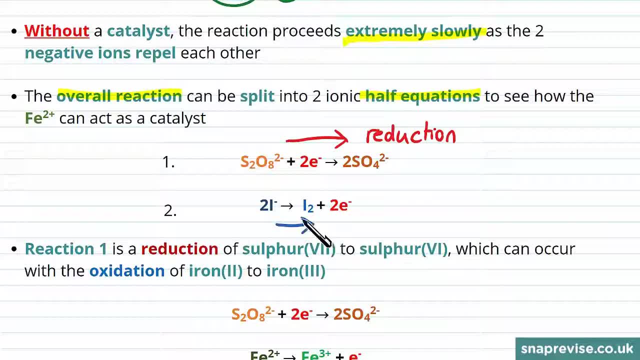 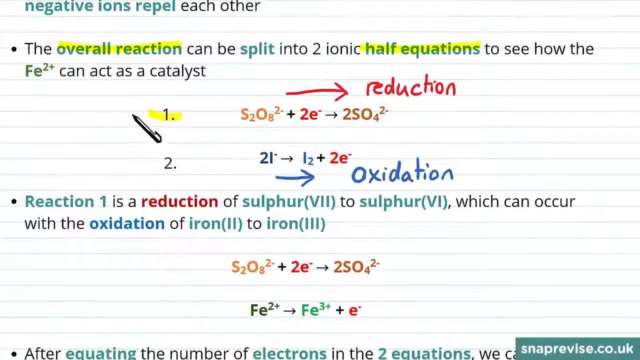 we have the iodide ions losing electrons. so this is oxidation. So we can use iron to make reaction 1 happen, because the iron can be oxidised from ion 2 to ion 3, and if we write the half equation for that, then we can get a reaction of zinc and iron 2 and